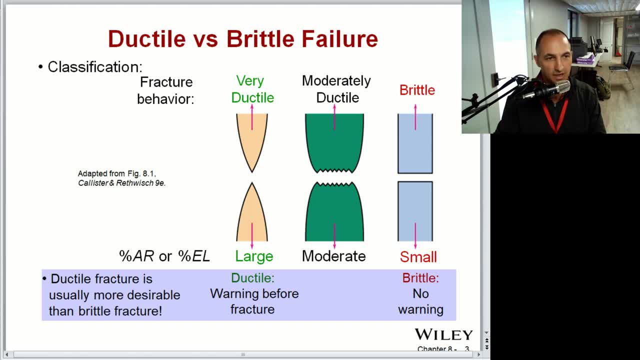 your material than with brittle fracture ductile versus brittle failure. there is three classifications here for fracture behavior. have a sample that is very ductile and you have complete necking and a point here at which it breaks. have moderately ductile sample sample, where you have some amount of 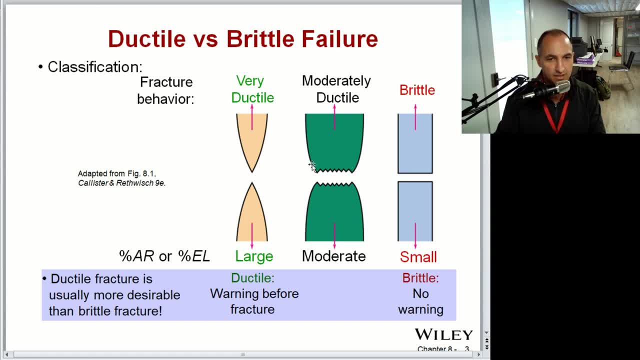 necking and then failure. that has a very fibrous surface and with brittle fracture you have no necking and a very flat fracture surface. to quantify the degree of ductility, we use there the percent reduction in area or the percent elongation, and those were equations that we discussed. 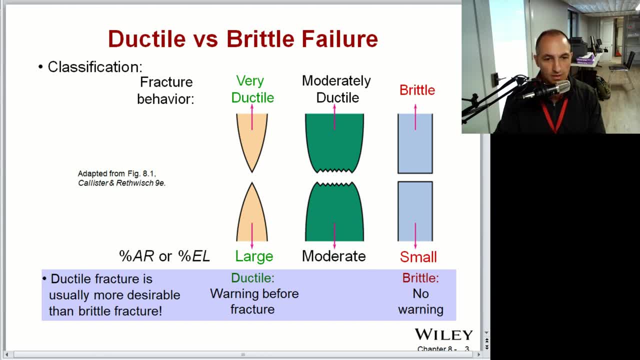 it in previous chapter. so for a ductile fracture it's more desirable than a brittle fracture because brittle fractures have zero warning before failure and for ductile fractures typically you will be able to see a small crack or it catastrophically fails a moderately ductile sample. 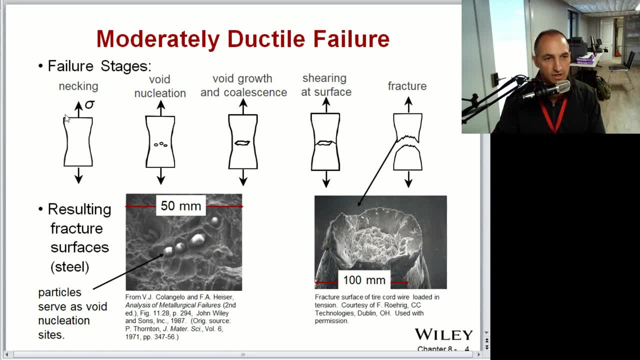 that was the one in the middle. you start to get some necking when you apply pencil. stress, start to get void formation internal for the sample and those voids gonna coalesce and you get sheering for the hole in the sample and her Mongolian nail failed, or 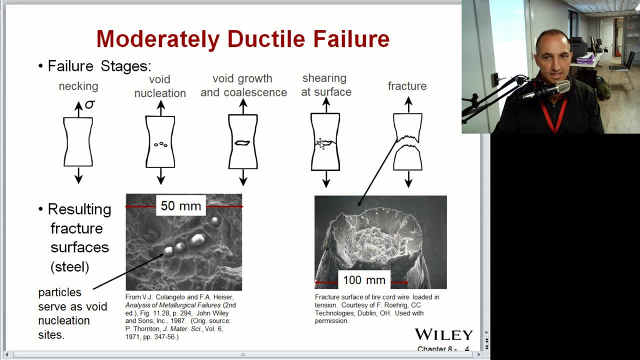 sans أنہAr communications. as always, 3dp cordless razor and 3d-ah P sprechen right at these surfaces here, here, followed by fracture, and if you were to look at the, the voiding areas, you might be able to see some particles, and these serve as nucleation sites. 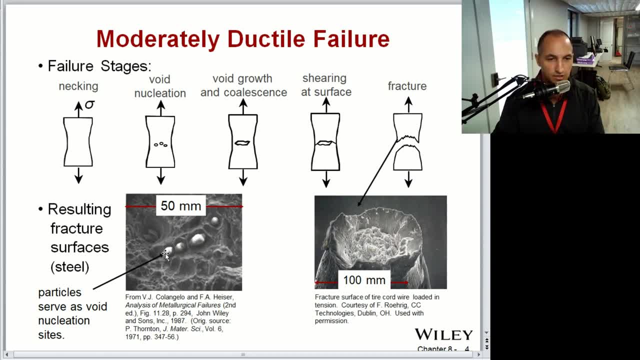 these particles might be small inclusions or slag or another precipitate in there and this is a specimen here- under some sort of high magnification and at fracture. you look at the surface here you'll see like a fibrous interior and then these sheer lips again. 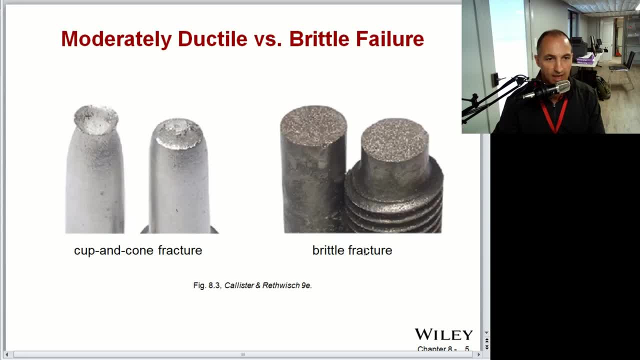 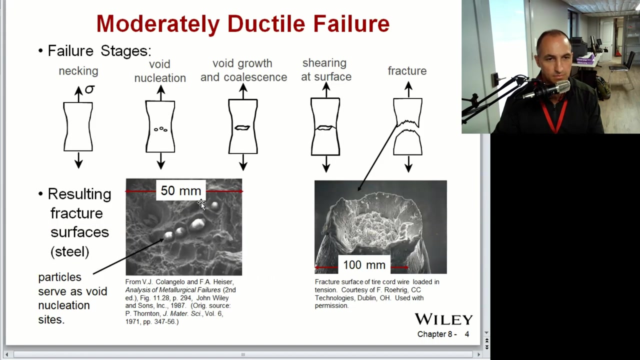 we call them around the edge and on the left we have a ductal sample and that has the sheer lips. we call this a cup and cone. the cup is on the left and the cone is on the right and that was the other surface of the same sample and a brittle fracture has a very grainy. 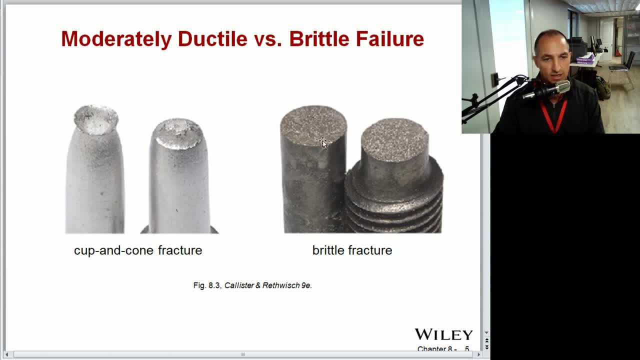 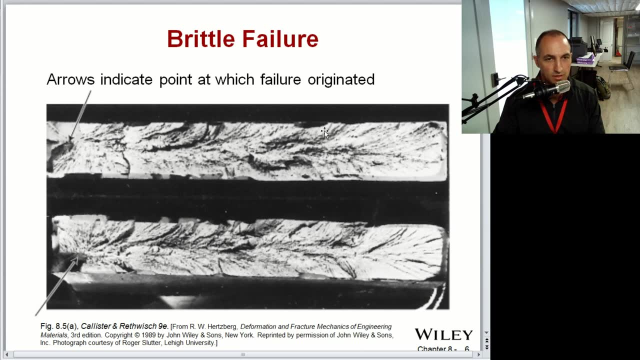 surface very flat and no necking. this is a sample with brittle fracture and you have what we call here chevron marks and these are like a almost like arrows here, and these are pointing- always point towards the initiation of failure. so in this case the arrow is pointing some sort of 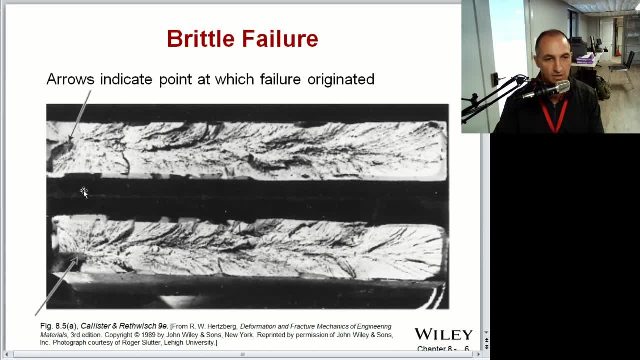 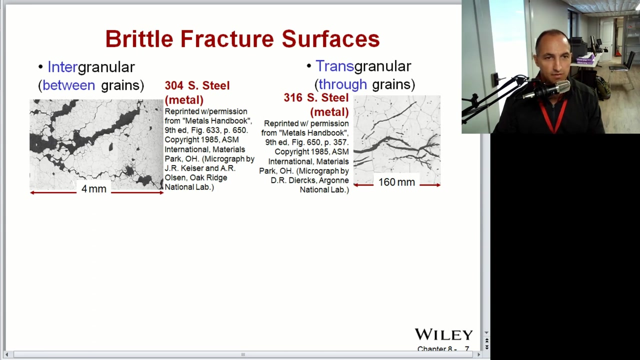 inclusion or a slag where the failure initiated. great for failure analysis and, like forensic analysis, to determine what was the cause of failure. here are some micrographs of a brittle fracture surface. sometimes in a brittle fracture you will see intergranular cracking, which that it cracks along the grain boundaries. that's intergranular. 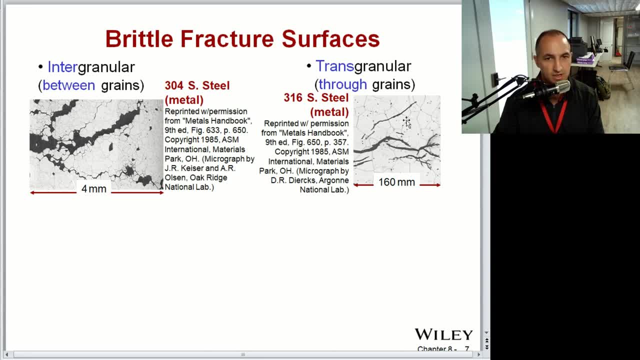 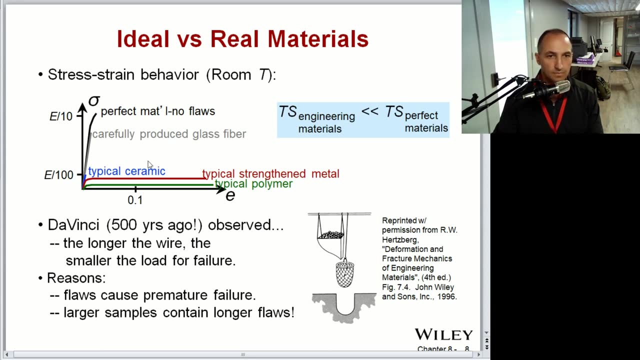 this is a 304 stainless steel sample and on the right you have transgranular fracture where the cracks are going right through the grains. this is a 360 stainless sample. all right, so this is ideal versus real materials. the stress strain behavior: stresses on the y-axis, strain on the x-axis for a perfect material with. 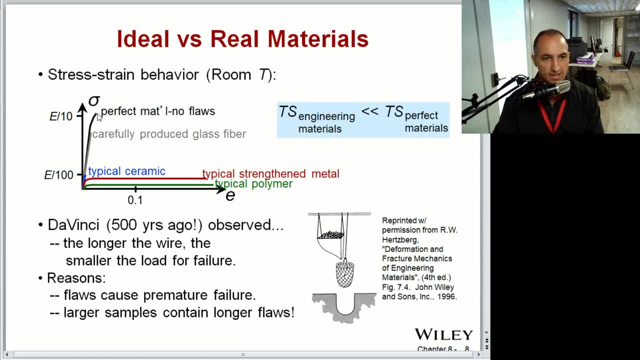 absolutely no flaws. might have a yield stress up around a 10 of the elastic modulus or carefully produced glass fibers. it will be slightly less but and not a perfect system and for a typical ceramic will have some around elastic modulus divided by a hundred for the yield strength and 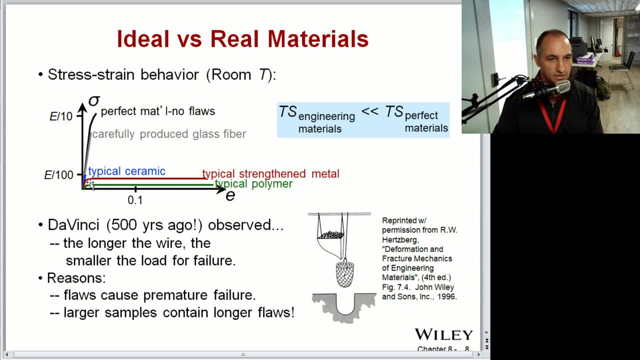 typical strengths. typical metals are in red here and a typical polymer green. so, definitely, engineering materials are going to have tensile stresses much, much less orders of magnitude less than what you would have in a perfect crystal. so what is this telling you? what's telling you that the reason why we have failure is because of the imperfections that are? 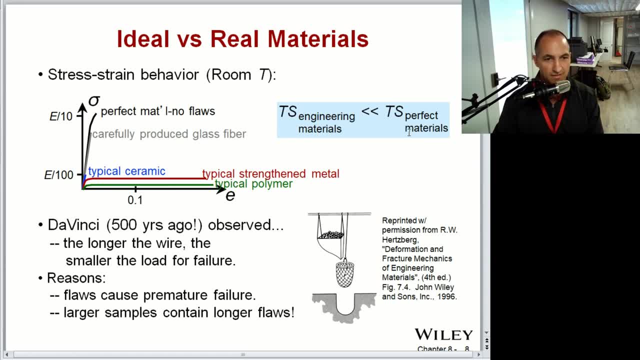 inside of it, and da Vinci noticed this over 500 years ago. he took a long wire and he hung some weights by it, and what he noticed was is that the longer the wire, the smaller the load, for he had failure, though there's a probability of having larger flaws when you have a greater or larger 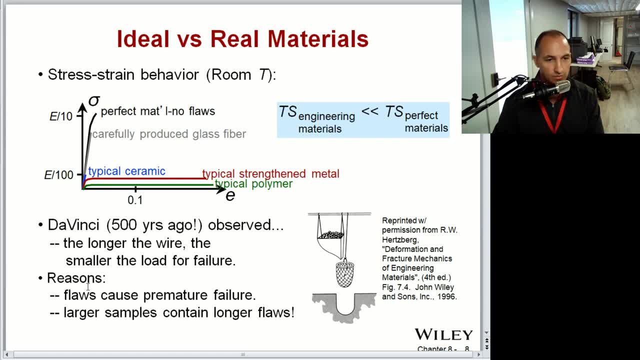 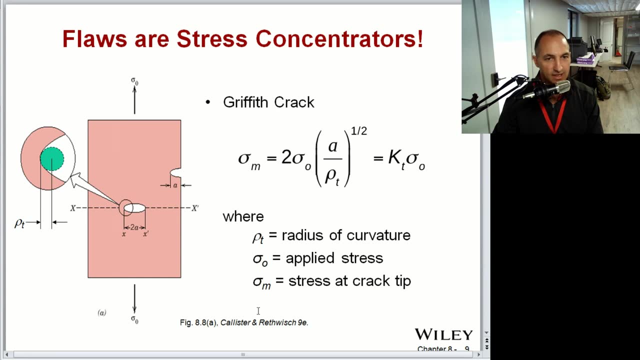 sample. so the reasons our flaws cause premature failure and larger samples contain larger flaws. so we have a Griffith crack here- that's what we call this- where there is a internal crack, or we could have a surface crack, and the equation is Sigma m, which is the stress at the crack tip, is equal to 2 times stress, that's. 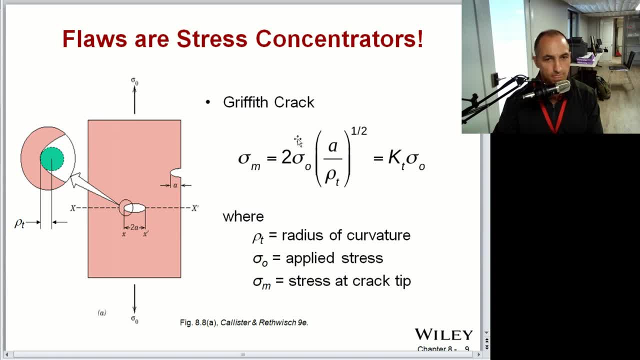 applied here, which is the externally applied stress times square root of A over Rho. now, a is the crack length, or I should say half the crack length, and Rho here is the radius of curvature. so this is equal to then KT, Sigma naught, and K is the stress concentration factor, if you. 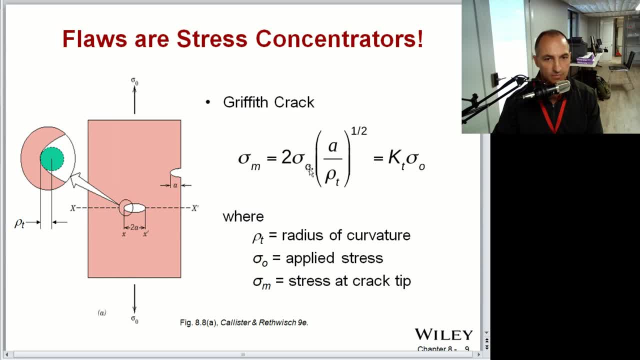 were to just take all these constants here, not constants, but if you were to take Sigma M over, Sigma naught at the stress concentration factor, as you can see here that if we increase the length of the crack, which is a, we're going to have a higher stress at the crack tip. 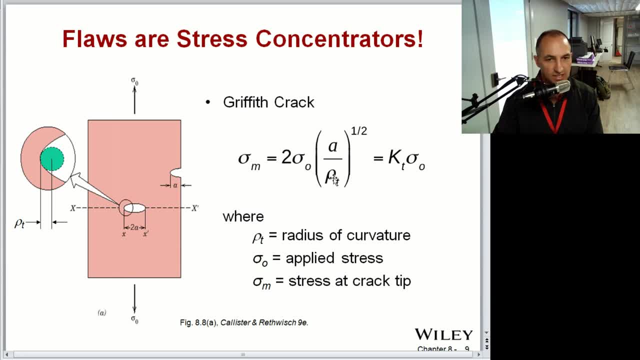 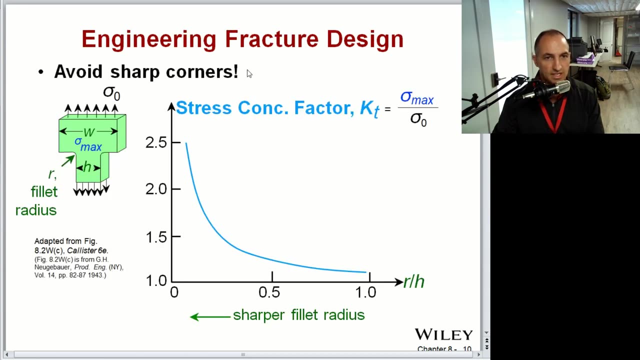 and if we decrease the radius of curvature, which is a sharper crack tip, you will also see a much higher stress at the crack tip. you engineering fracture design, something that's important for all of you. what we need to do is we need to avoid dark corners. here is a specimen where we have a sample, where it's wider at the top, it's: 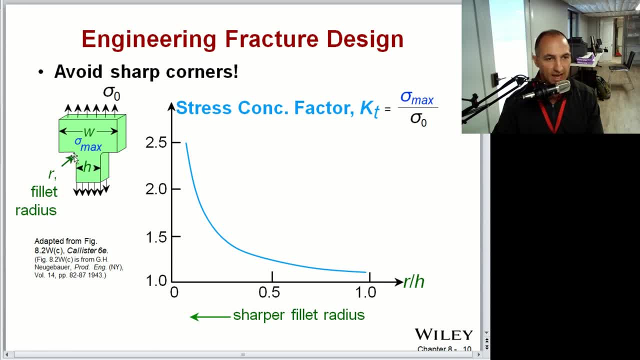 in here in this area and we're going to have a stress riser or stress concentration at this corner here and the more we can round out that corner, the lower the stress is going to be at that at that stress concentrator. this graph here of stress concentration factor KT versus a radius of the crack: 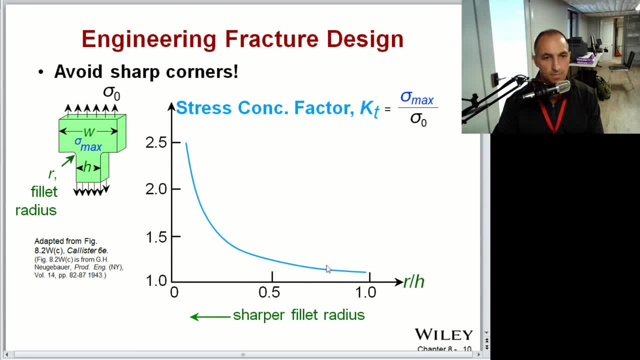 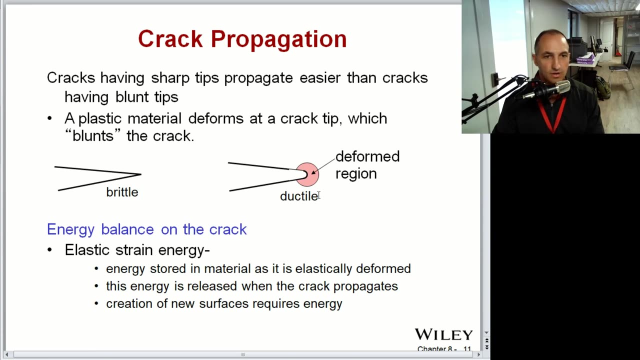 or radius of curvature of a sample. and then we're going to have a stress concentration factor, KT, and we're going to have a stress concentration factor for this one. so we're going to have a stress the same for this one. so we're going to have a stress concentration factor that's going to go up. 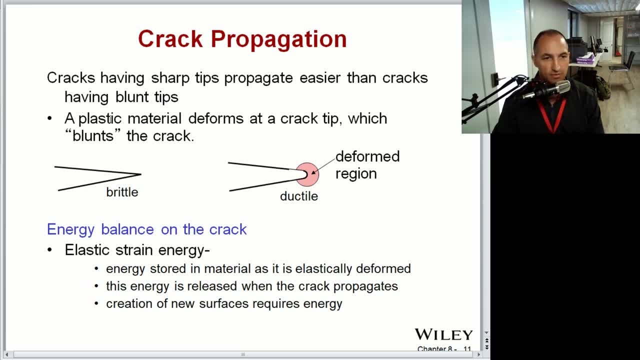 exponentially at the bottom of the layer. in line with this example, stress concentration is going to go up exponentially with a smaller R over H. having a sharper tip propagate easier than cracks. having a blunt tip. saw that from the Griffith equation as well. so a plastic material will have deformation. 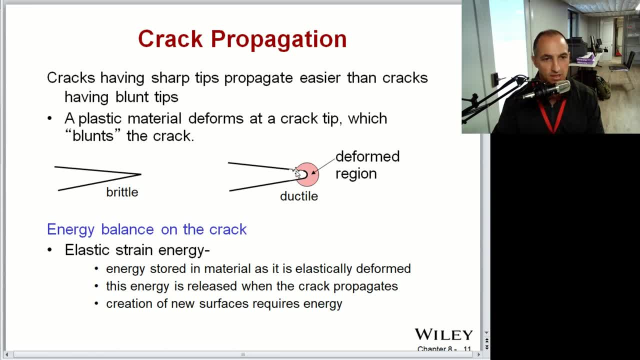 at this crack tip and that leads to a blunting of the crack tip and this is an area of deformation because it is the highest stress in the sample. now there's an energy balance on the crack, where elastic strain energy is the energy stored in the material as it is plastically deformed and the energy 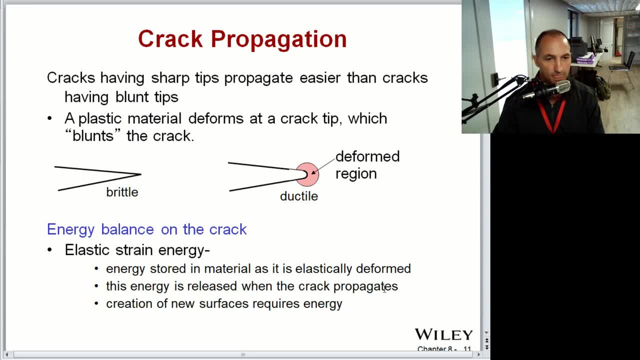 is released when the crack propagates and then you have creation of new surfaces which require energy. so the energy from stretching of the bonds during the crack is released, and then the energy is released from the crack during the elastic strain is then released immediately when it cracks and 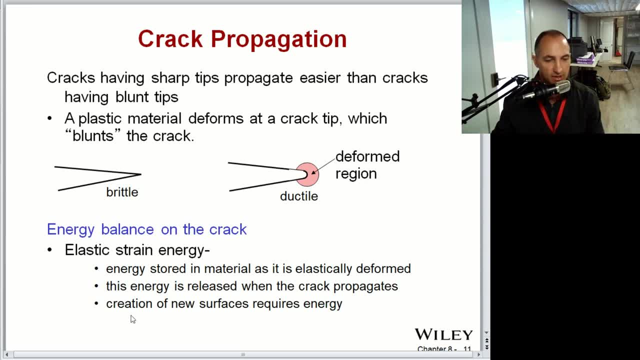 that release of energy is. some of it is transferred into the creation of new surfaces, because this crack is going to propagate further and also you're going to have some release of energy, some of it really. energy Hooke's law is something that we can refer back to here, where force is equal to the force of energy. 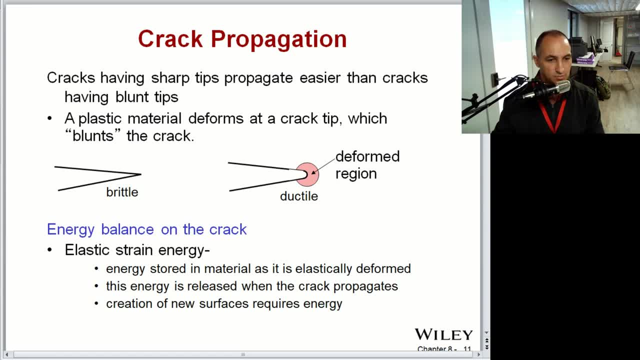 the force flows through the form of a mu codeque, and so we don't California set it on to its own, we like to call it linear. so this particular case we call it linear, and this particular case we call it linear because this is the fluid vais getting. 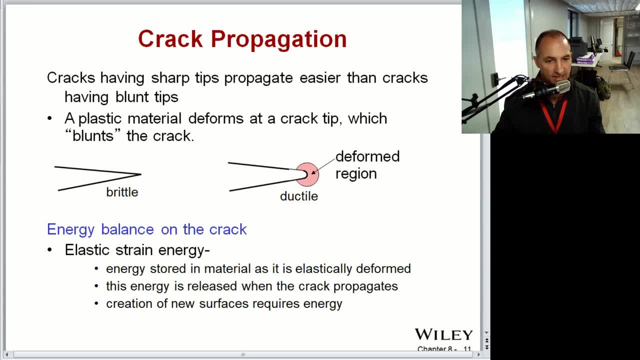 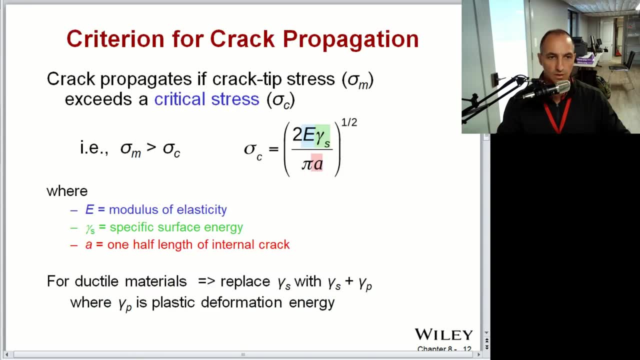 over into negative and negative and negative. and here, at this point there's no, and this is the guy illustrated between Nobel andski. I'll just go through all of where. K is the spring constant, X is the distance criterion for crack propagation. the cracks will propagate if the crack tip. 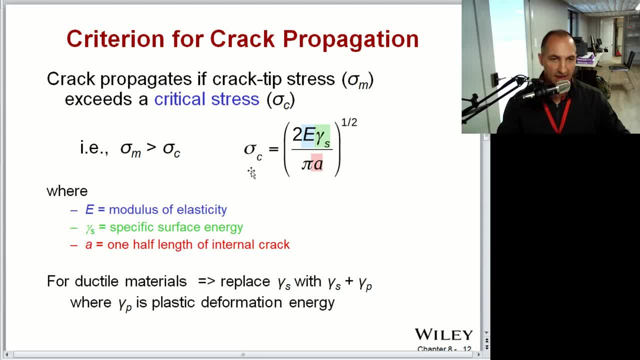 stress. Sigma M or Sigma max exceeds the critical stress. Sigma C. equation for the critical stress is two times the elastic modulus, times the specific surface energy over pi times half length of the internal crack and the square root of that will give you your critical stress. this is the equation for: 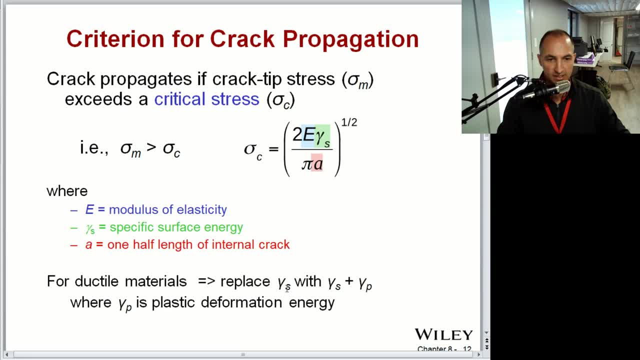 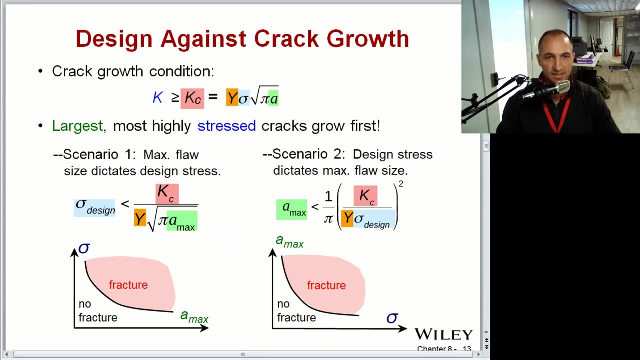 brittle materials. so for ductile materials you want to replace gamma s with gamma s plus gamma p. we need to design against this crack growth. so crack growth is going to be crack growth when the fracture toughness a is greater than K sub C. that's your critical. 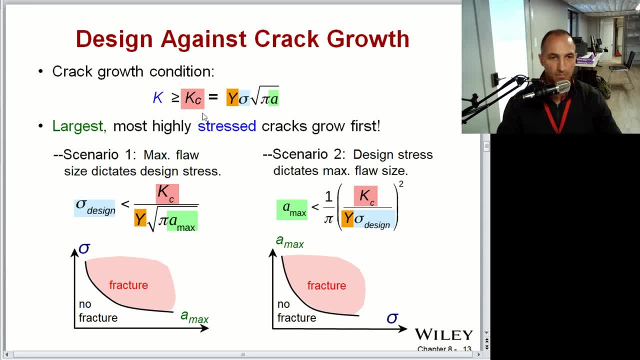 fracture, toughness, and this is a property of the material. so that is equal to Y, which a dimensionless parameter, which is a function of the crack and the specimen, dimensions and geometry. and look up Y values in tables in your book and this is your stress: times: root pi. 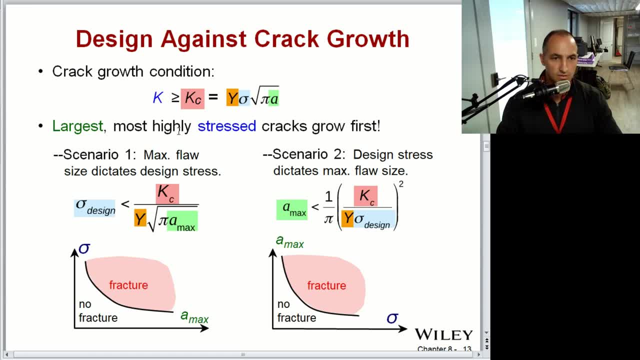 the most highly stressed cracks are going to grow first. we have two scenarios here. one is an example where you would have crack detection equipment that has a minimum resolution to find cracks. in scenario one, the max flaw size is going to dictate the design stress, so we'll need to send this design stress. 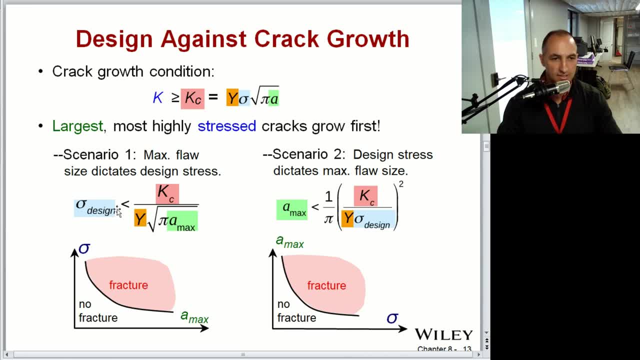 back to the engineers and say this: you need to design this aircraft or whatever, to not exceed that value. now, on the other hand, you might have situation where you have no choice but to accept the stresses that will be placed on on the design. you better have your crack. 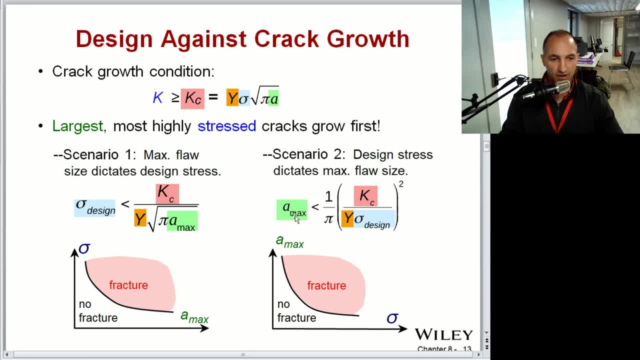 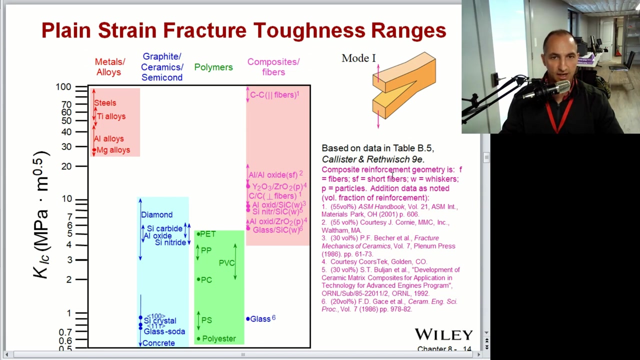 detection equipment that can find cracks that are as small as your A-max here. you do not want to be in these red zones here. for scenario one: you do not want to be in these red zones here. or scenario two: here's a table of plain strain fracture toughness ranges just to get you up to. 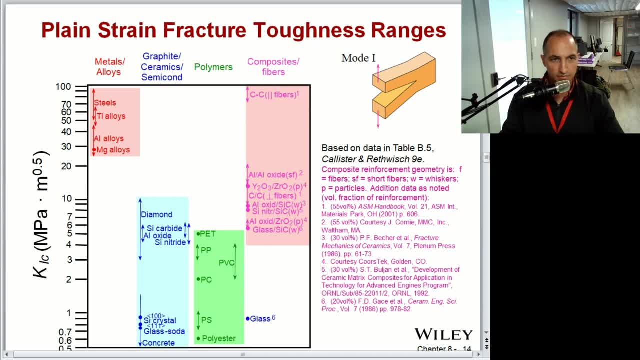 speed. here there's different modes of fracture toughness. this happens to be mode one. there's mode two and mode three as well, and those just mean that the sample is, instead of being pulled apart, it might be sheared or torsional. so there's different modes of stress on this crack, so this happens to be mode. 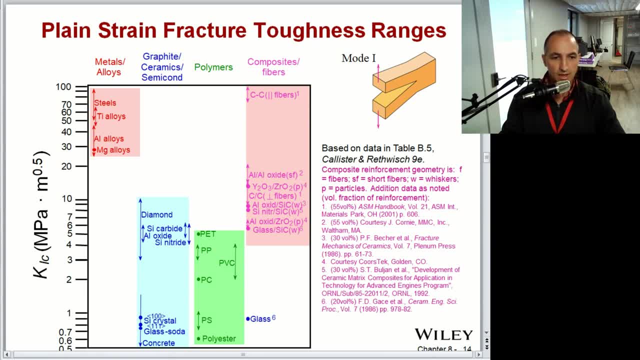 one. but there's also this new term here, which is plain. now, the plain strain is when the sample is thick enough that we can ignore any lateral strain, that we can ignore any lateral strain which are perpendicular to the force acting on it. but it's you know thick enough here that the bulk of the material is stopping any. 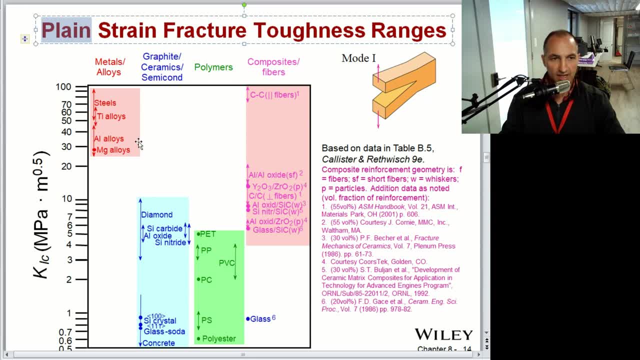 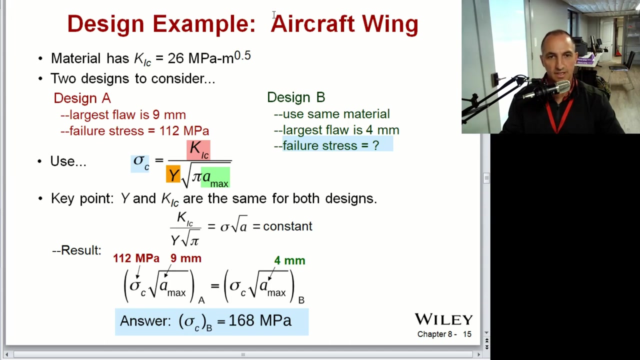 lateral strains and here we can and look up values of a1c or plain strain mode one, plain strain fracture toughness for different materials and we can use that as a part of our design- determine what type of material we need to use to for our specimen. here's a design example for an aircraft wing. this happens to be aluminum alloy. 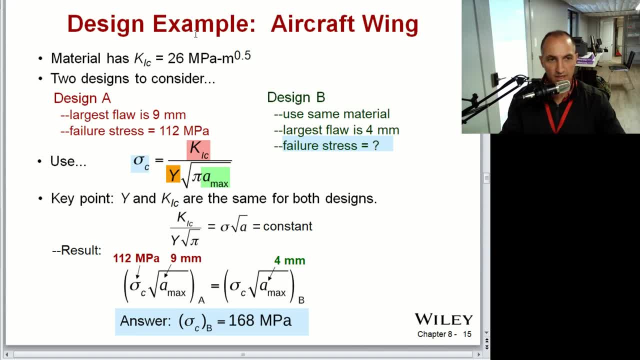 which is what they use for aircraft wings normally. it has a plain strain fracture toughness of 26. there are two designs. consider for this wing design A and design B. design A: the largest flaw that is allowed is 9 millimeters and the failure stress is 112 megapascals. 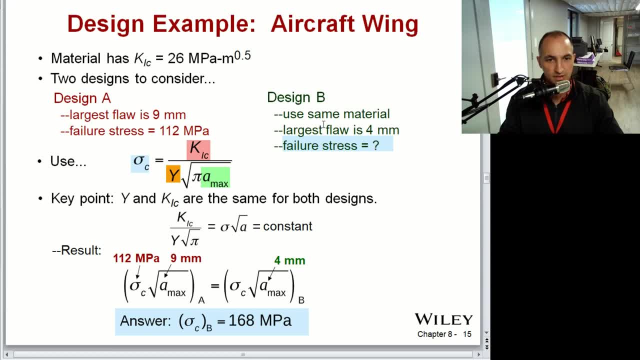 and the question here is: is: using the same material and where you can only have a flaw of 4 millimeters, what is the fracture stress allowed for that sample? so we use this equation: Sigma C is equal to fracture toughness over this Y, which again is your dimensionless parameter, times the square root of pi A. 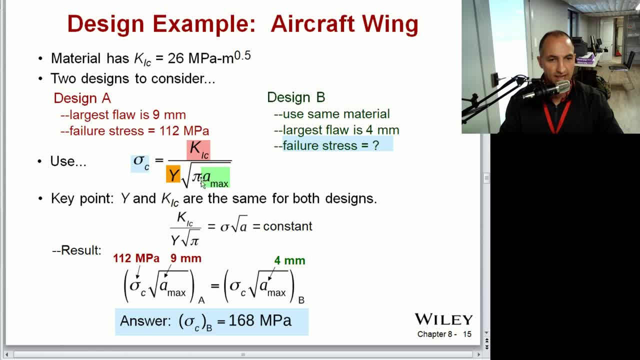 and remember A is just half the crack comma. you can't go through this with a number that's not quite the same way length and we're not. we are not provided with Y, but we don't care because it's the same for both designs. so if we make 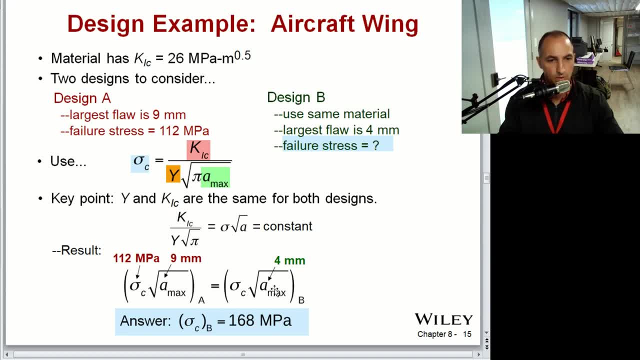 this constant. here we can just equate the two together, so we know the design stress and the length of the crack which is allowed, and then just solve for Sigma C, for the B design, and we get a hundred and sixty eight megapascals. so that is the failure stress for design B. 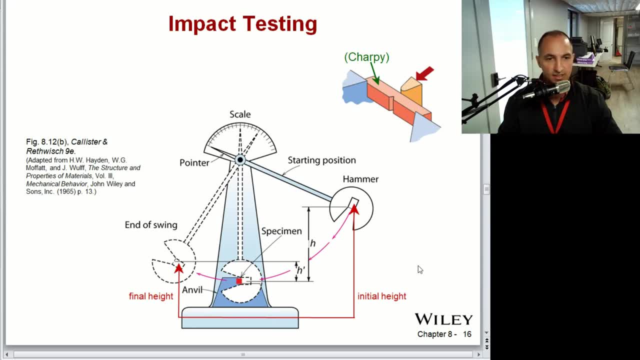 one of the ways to measure the toughness is to measure the length of the crack which is allowed and then just solve for Sigma C, for the B design, and we get a hundred and sixty eight megapascals so of a of a sample. here is with this impact testing and this is just a giant. 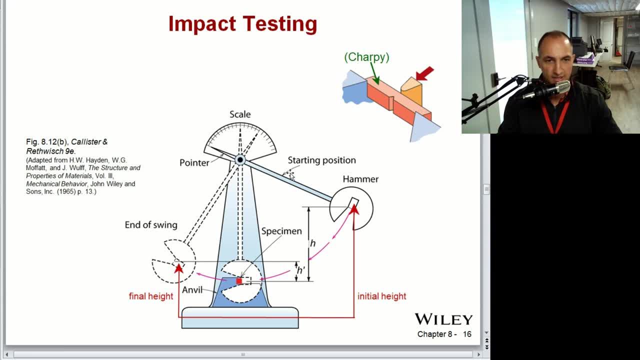 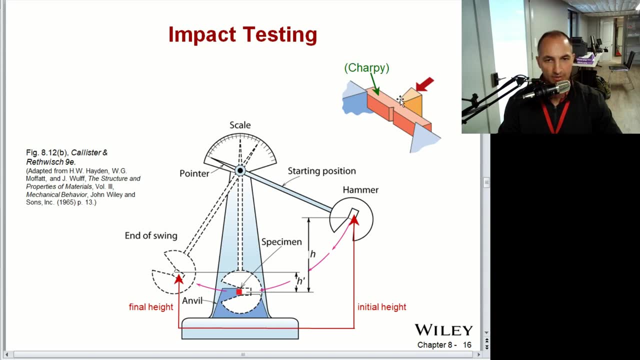 hammer with a huge weight on the end of it and it's dropped from a from a certain height and it swings down and it slams into the sample and then it swings up to a final height which is going to be less than the initial height. your potential energy is M. 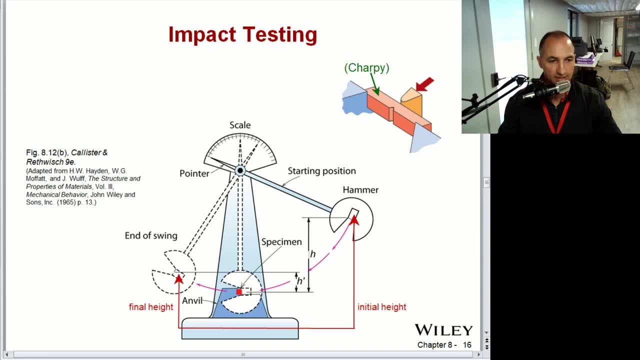 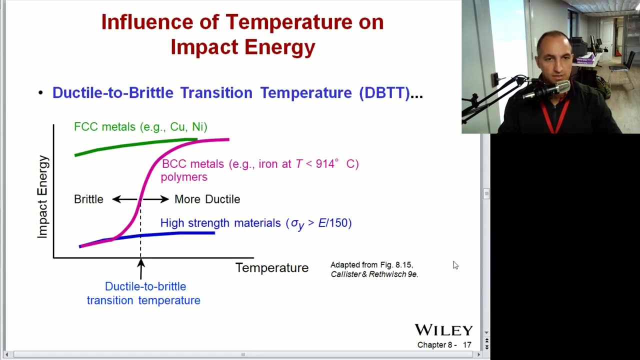 G, H, remember from your physics class. so it's M G times the change in height. but the energy absorbed is the difference in the potential energy of that hammer from the initial height to the final height. the influence of temperature on impact energy in a lab that I did in my. 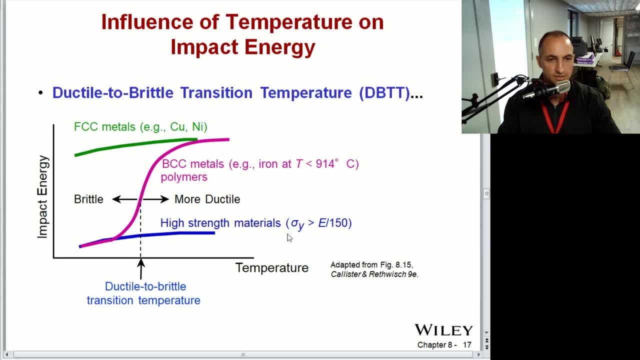 engineering courses we took different Nope which was less than M Sharpie samples that you saw previously course that you did in your층 and we would eat those or cool them down and the plot points of that impact energy versus temperature of the sample. what we found is that for BCC metals 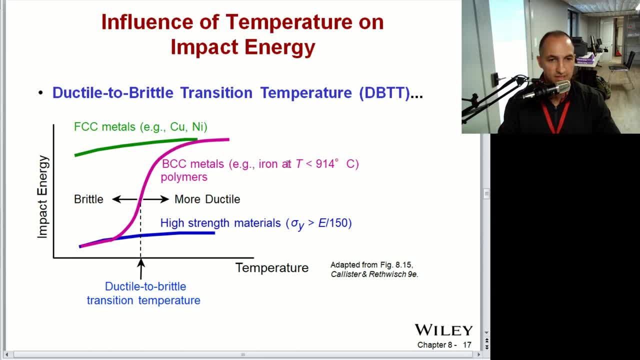 which are the Ferris metals like iron And up against出來 some polymers. they have a ductile to brittle transition temperature where it will become very brittle at low temperatures and become ductile at high temperatures. FCC metals don't exhibit the ductile to brittle transition and 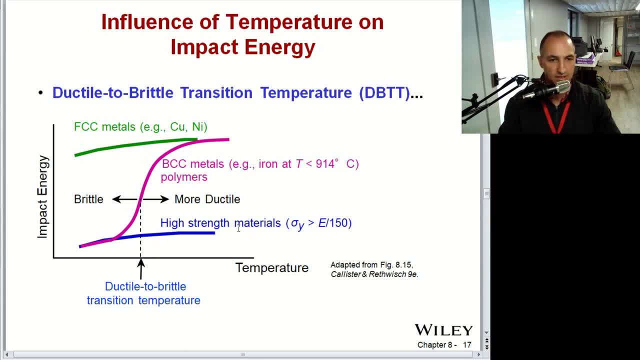 also high strength metals don't experience those either. however, the impact energy for high strength materials is very low anyways, why do we have this transition for BCC metals but not FCC and high temperatures? I'm sorry, high strength materials. so we will discuss the answer to that question. 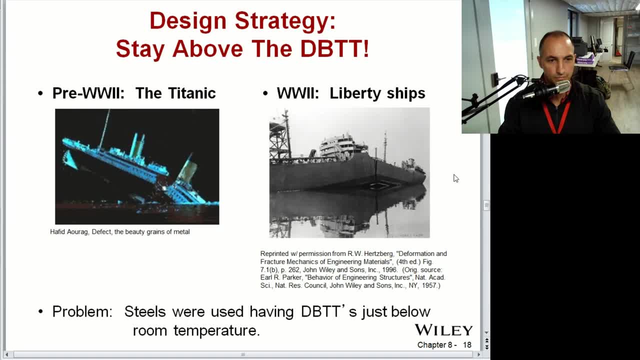 class. there are some stories in our history book that taught us some lessons about why we want to be very, very concerned about the ductile to brittle transition temperature. on the left is the Titanic, and Titanic always fascinated me as a kid and I read lots of books about it and I was very much interested in what really happened. so 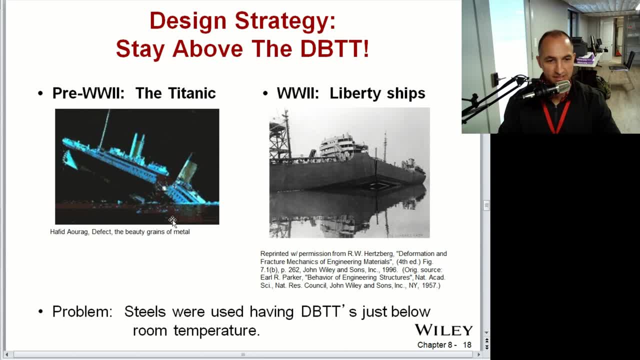 well, did it break in half on the surface, as as we saw in the movies and and read in the books, and there is a analysis of the Titanic sinking from samples that were brought back when they filmed IMAX and they went down back in 1991. 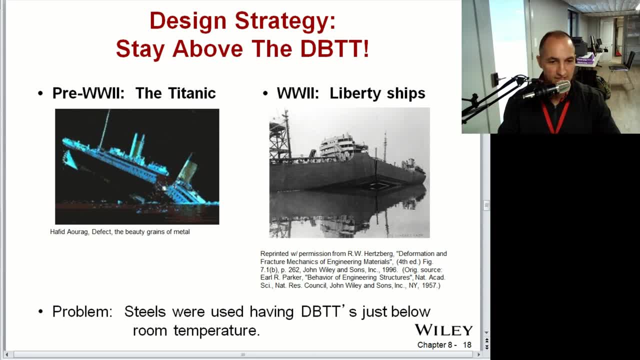 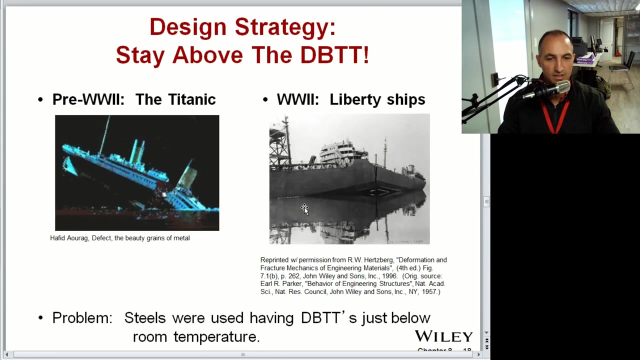 they're filming the movie and what they found is that there was 100% brittle fracture and it had to do with the cold water temperatures where the Titanic tank and it was about 28 degrees fahrenheit when it sank- on the right we have the World War, two liberty ships, and all these liberty ships started breaking. 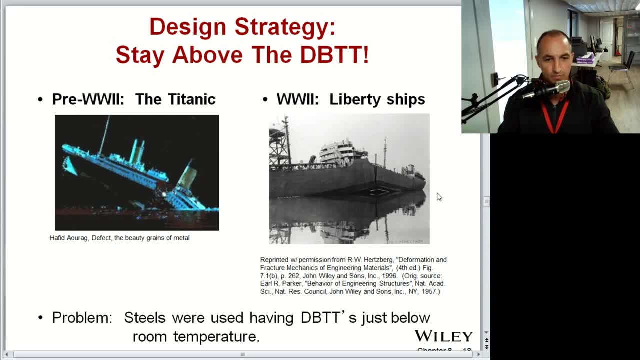 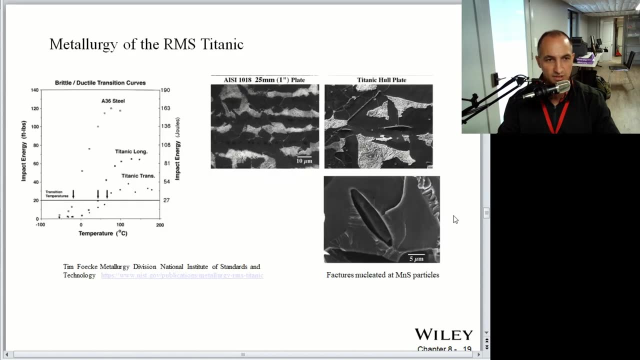 in half right around the centerpoint here. a whole bunch of this happened to a whole bunch of the ships. again it was a bcc fields that were below the ductile to brittle transition. i recommend that you go to this link here, or this national institute of standards technology. 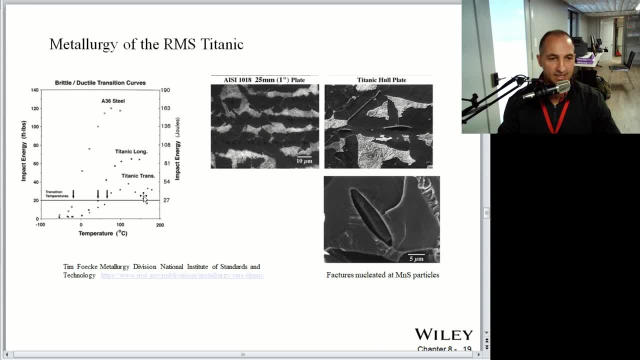 where they published the results of the titanic, and here's just a quick summary of their findings. the ductile to brittle transition of modern a36 steels is approximately 25 degrees celsius here, but for the titanic it had a ductile to brittle. 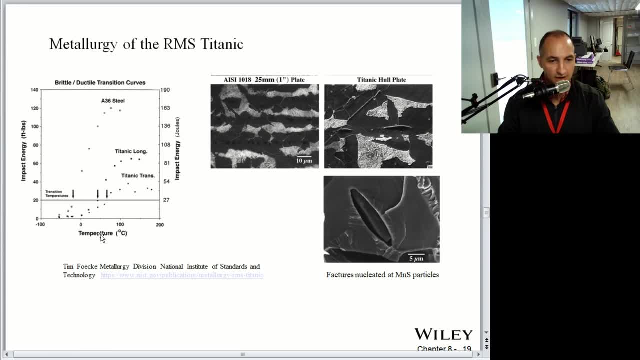 transition of around 40 plus 45 degrees celsius, which is, uh, much higher than the temperature of the sea water when it sank, which we estimate to be was somewhere around negative two degrees celsius. so modern steels would have been fine, um, but not titanic steel. so this is differences in. 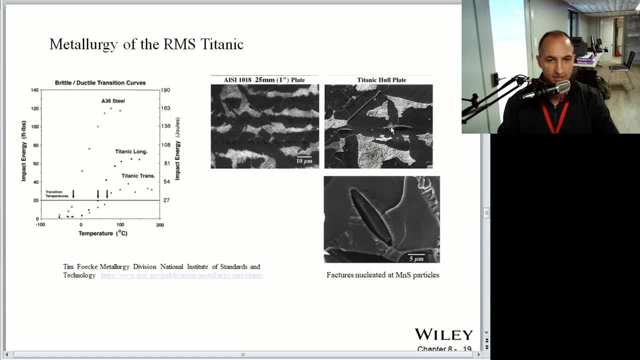 micro structure between the titanic hull steel and modern steel. here on the left, grain sizes were bigger, the pearlite was much finer here and all of these and you with. there were also these particulates of magnesium sulfide which were points of initiation for failure. there were a few other findings as well, which you'll 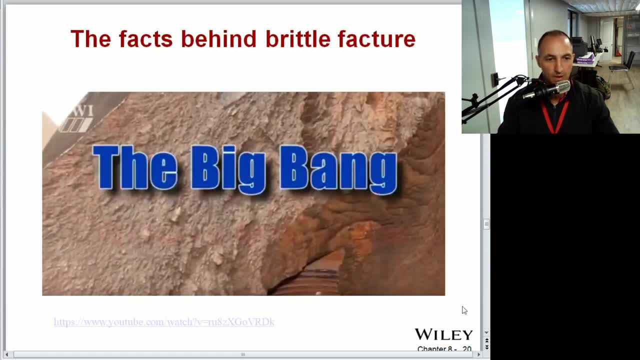 see in the article. next, i'd like for you to watch this video called the big bang and i will play it here briefly for you, or just the first start of it, but i would highly recommend that you go in and watch this video. bring it up here. 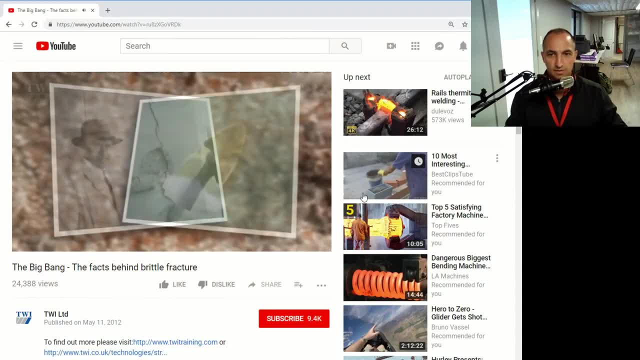 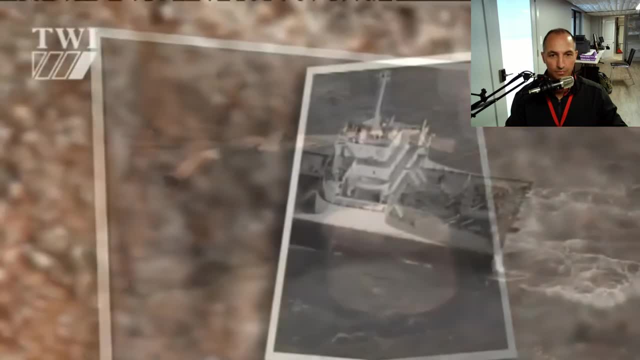 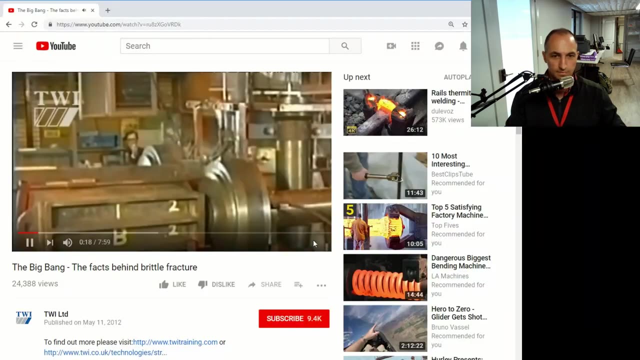 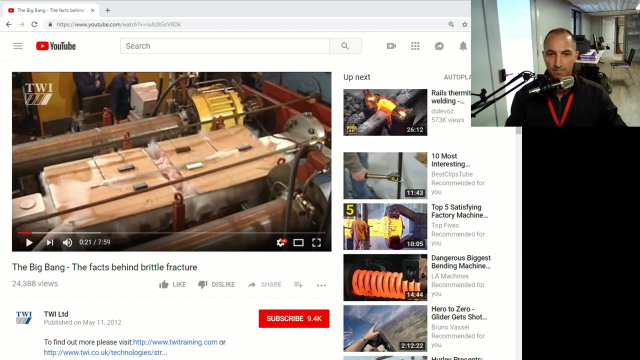 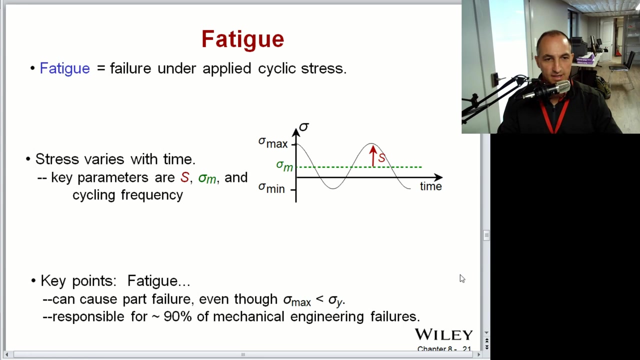 and this my own chord, all right, so please go ahead and watch that, have time, and on with the presentation. there's another phenomena here with failure, which we call fatigue. a fatigue is failure under applied cyclic stresses. fatigue is responsible for 90% of the mechanical engineering failures that we have. that's a huge, huge problem, and 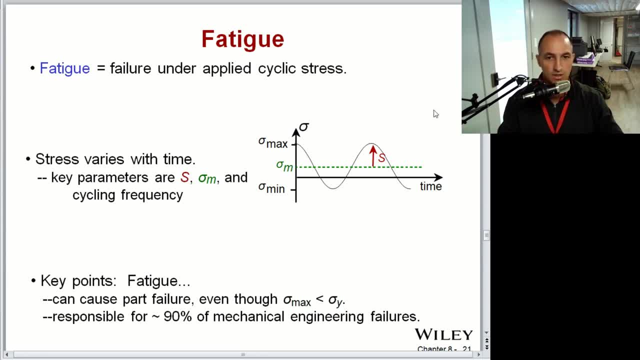 something that you cannot ignore when you're designing structures or or whatever. so the stress varies with time and it's a sinusoidal around some nominal value of Sigma M, and so S is just the amplitude of stress frequency, and so, interestingly, you can get failure. so you can get failure of your. 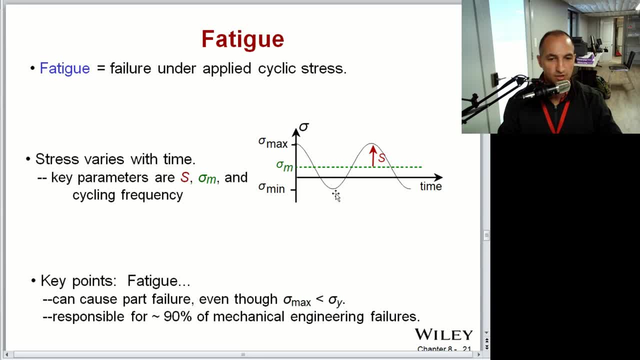 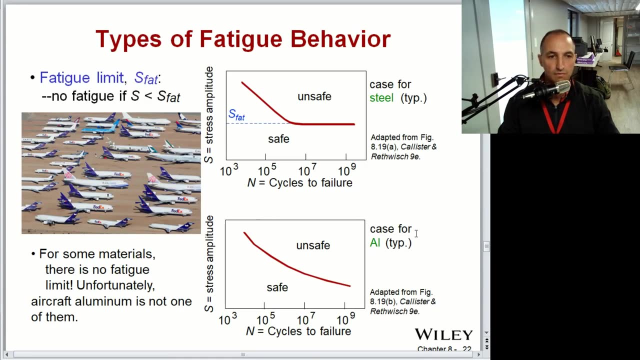 part well below the yield point of your sample. so Sigma max is less than Sigma Y or your yield strength. this is obviously a big problem for aircraft. you've heard stories of, you've heard stories of the cabins ripping apart in flight at no particular, for no particular reason. 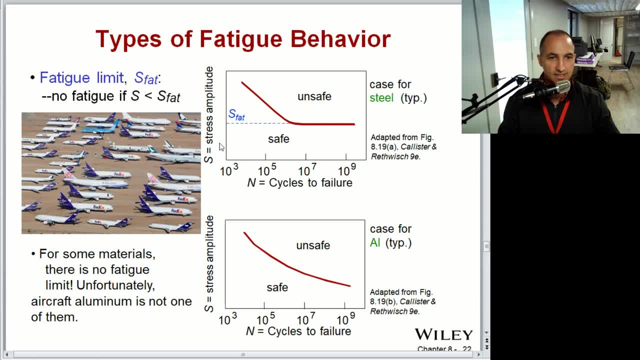 until they find out later that they didn't put that aircraft out of service soon enough. but there is a fatigue limit and if you are working with, like steels in you know, ferrous materials that have a fatigue, that don't have a fatigue limit, if you operate them below Sigma of f and if as long as you're here, you can you. 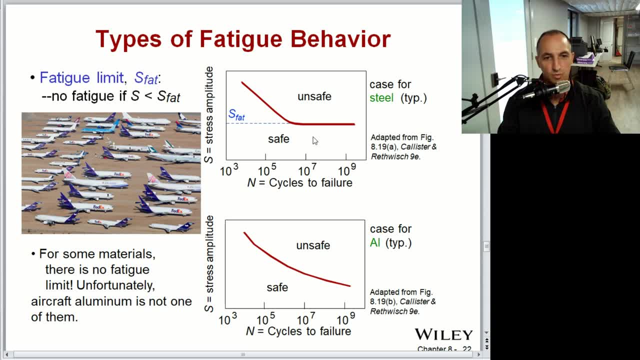 can cycle that forever and you'll never have to worry about fatigue. but for other types of materials like aluminum, there is a particularấy: u sk eng azy laga vessel Knowledge. that'sってる isn't a fatigue limit, and that's a real bummer, because eventually you're going. 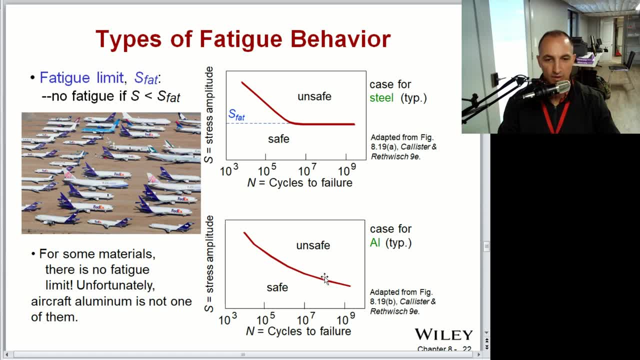 to have to put that aircraft or whatever out of service, as you're going to reach certain number of cycles here where it becomes unsafe, and that's why you have all these aircraft just sitting out in the middle of the desert here and what we call the boneyard out in the Mojave Desert- and I've been there before. it's. 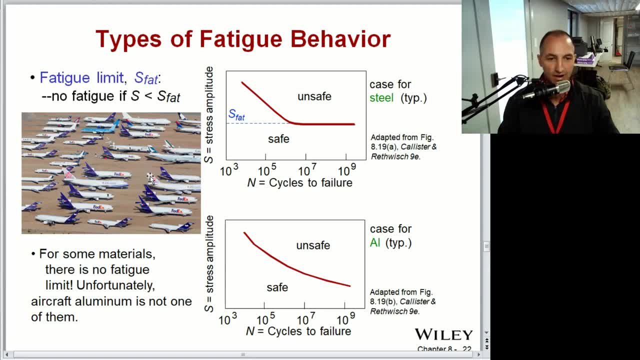 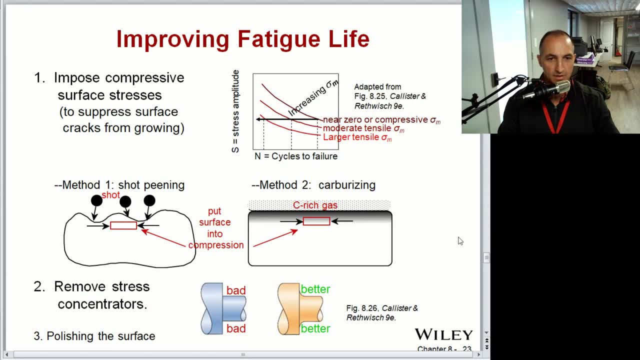 pretty, pretty amazing how many aircrafts have to be taken out of service as of that fatigue limit for aluminum. so to improve the fatigue life you do different things. one of them is to impose some compressive surface stresses, and one method to do that is with shot. 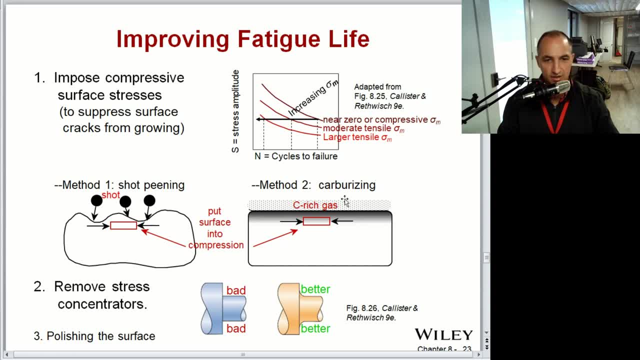 peening. another method that you can do is to do a lot of the same thing with the shot. peening- and that's another method that you can do is to do a lot of the same thing with the shot- is carburizing. carburizing is just injecting a carbon into the surface. that 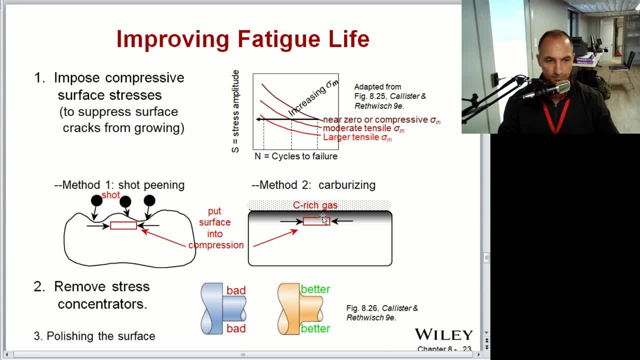 puts surface in a compression because of the carbon atoms that are being shoved into the interstitial sites of the host lattice. another another thing you can do is remove any stress concentrators, so you want to have fillets here- no sharp edges- and you can also polish the surface, as any scratches on the surface could be. 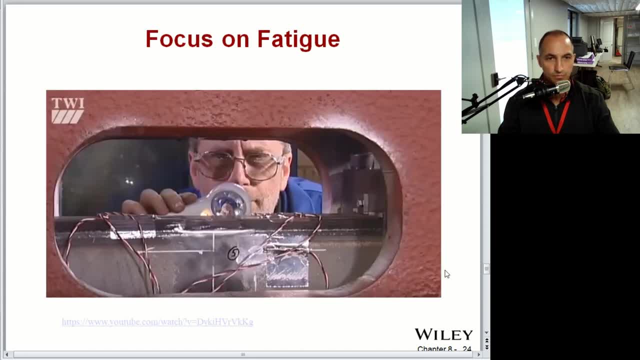 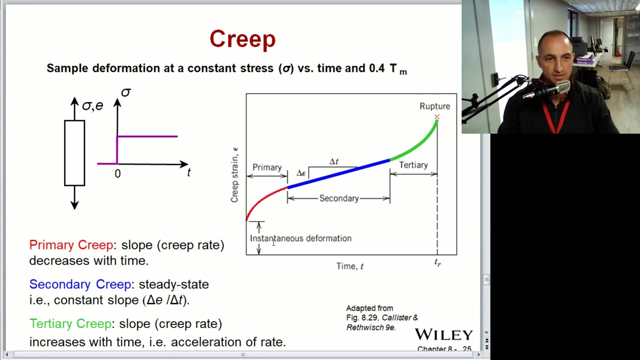 stress, concentrate. well, there's another video here which I recommend you watching, and this one has to do with fatigue. that's the same company that does testing on fatigue, and then the link to that is right down here. creep is another type of failure that materials engineers are concerned with. 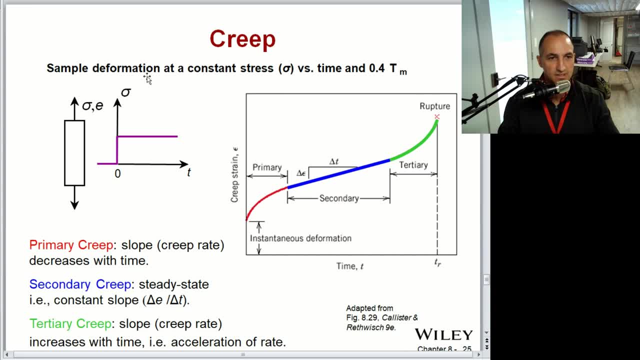 and a sample is as a deformation here at constant stress and we're looking at how it's straining with time and the temperature here is raised above room temperature. it's about 0.4 of the melting temperature and it goes through different regimes here where you have a higher strain rate. 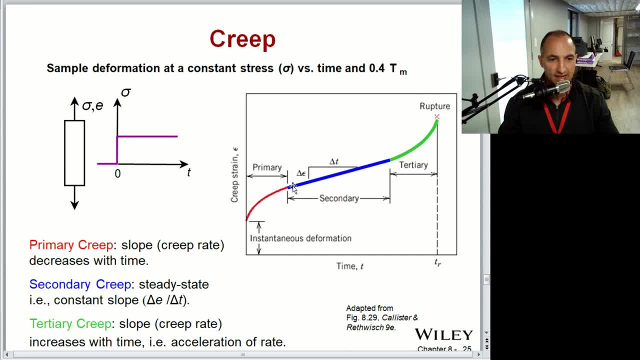 initially all the primary creep, then a steady state area of secondary creep, followed by tertiary creep where you get a much faster or accelerated rate of strain till you rupture. so why are we concerned about creep? and what applications are we concerned about creep? so it's any time the material is. 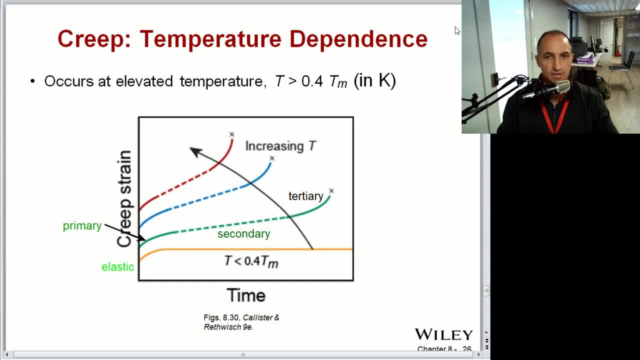 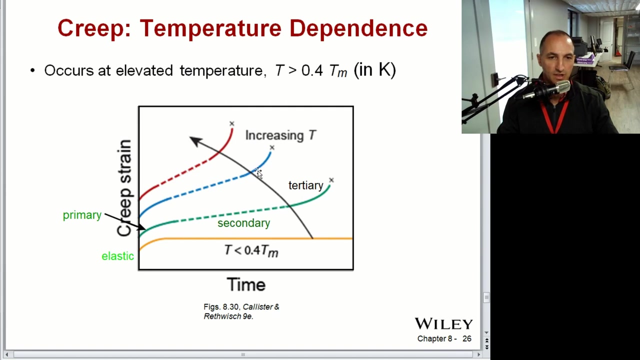 exposed to very high temperatures and for long periods of time, and here is a graph you're showing out. an increase in temperature results in higher strain and shorter time to failure. shorter time to failure with higher temperature. so the the yellow line here is that room temperature, and then green, blue and red. 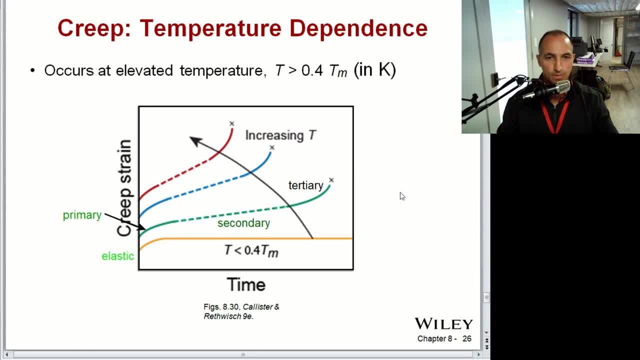 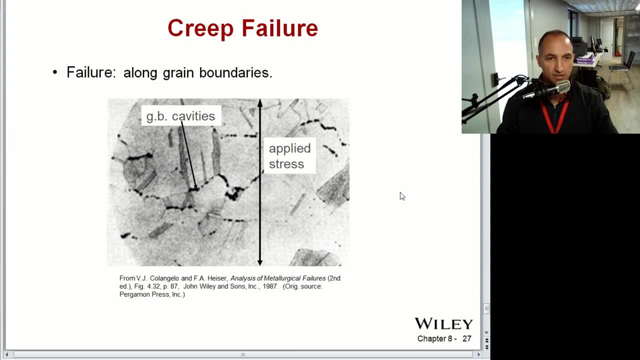 go to hire and higher temperatures, grape failure is will occur along grain boundaries, so you'll want to reduce the grain boundary area to reduce creep. that means larger grains or some extreme. you can have single crystal samples and that will have no or, you know, very little creep. for that reason, and that's why we often will produce. 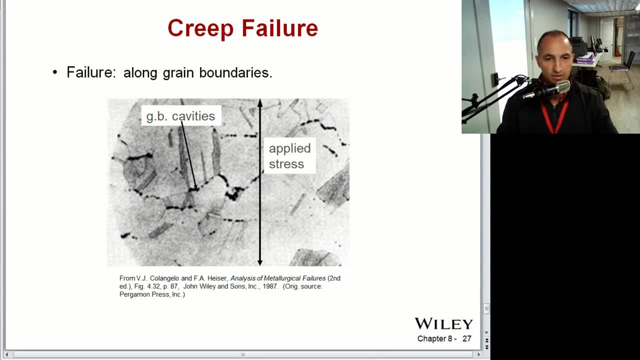 turbine blades out of the single crystal of metal. these turbine blades are exposed to very high temperatures and a lot of stress. you can hang a tank from a three inch turbine blade and bring it up to half the melting temperature of the material and you'll get very, very little strain during that sample. 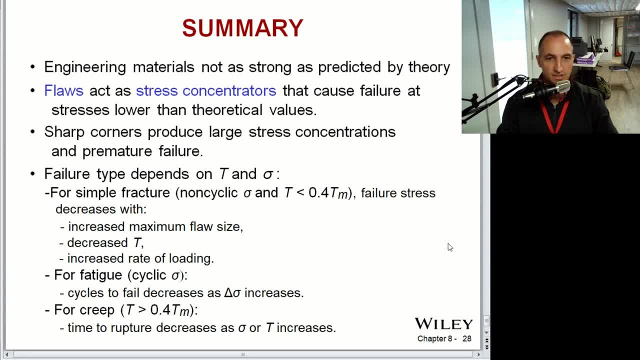 in summary, engineering materials are not as strong as predicted by theory and that's because flaws act as stress concentrates and that will cause failure. as stress is lower than the theoretical values. sharp corners produce large stress concentrations and premature failure. failure type will depend on temperature and the amount of stress: simple fracture, like the non-cyclic type, and when the